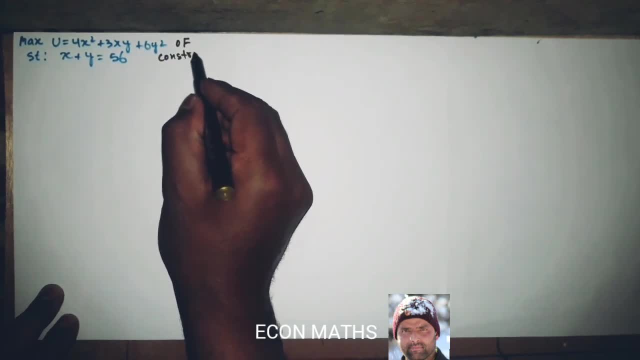 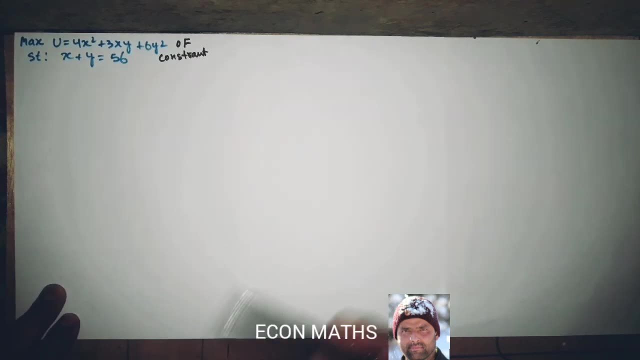 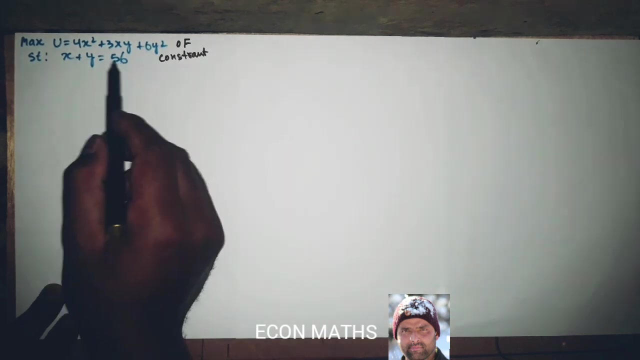 is the constraint. This is the constraint to this maximization. Now we have to solve this problem. Sorry, we have to maximize this problem. So how will we do this? First of all, we will set the constraint equal to 0.. We will set this equation equal to 0. So set constraint. 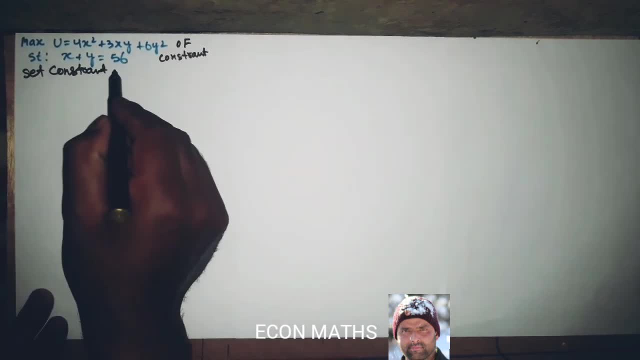 constant equal to 0. So this implies 56 minus transposing this will become minus x minus y is equal to 0. So first we set the constraint equal to 0. After that we will add the constraint equal to 0. So this implies 56 minus transposing this will become minus x minus y. 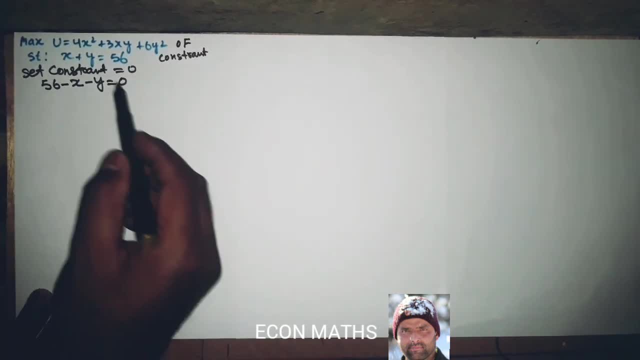 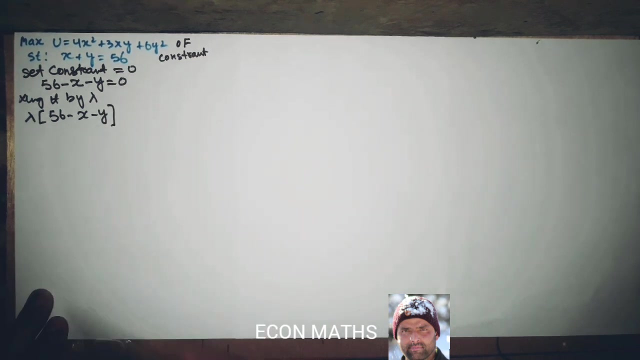 lambda. sorry, we will multiply this constant with lambda, therefore multiplying it by lambda, so this will become lambda times 56 minus x minus y. now, after that, to get the Lagrange's function, we will add this term to the objective function. so i will write: z is equal to. we will add this. 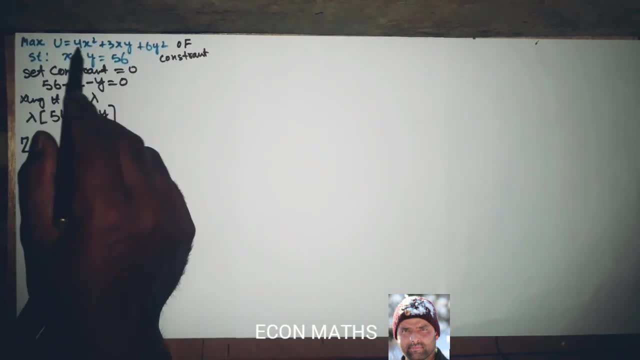 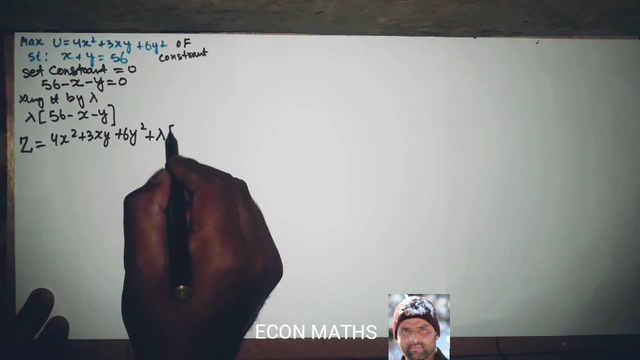 term to the objective function. so this will become- i will write first this objective function, that is 4 x square plus 3 x y plus 6 y square and i will add this term to this function: objective function. so here it is lambda into 56 minus x minus y. now to get the value of x, y and lambda we will. 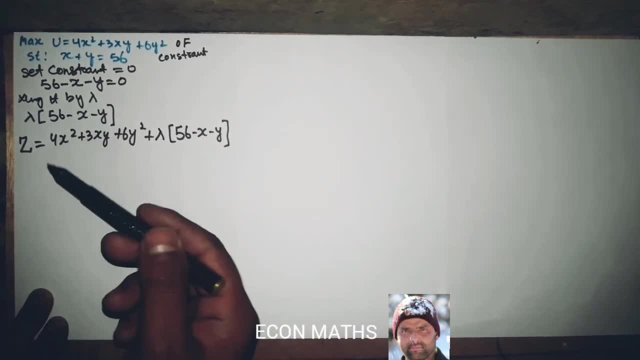 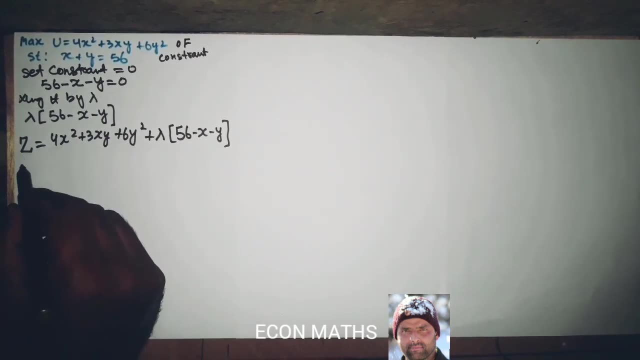 partially differentiate this Lagrange's function with respect to x, y and lambda. so partially differentiating. first we will differentiate this with respect to x, so i will write z. subscript x implies i am partially differentiating this with respect to x, so this will become now the derivative. this will become two fourths are 8, x plus here is x, so the derivative. 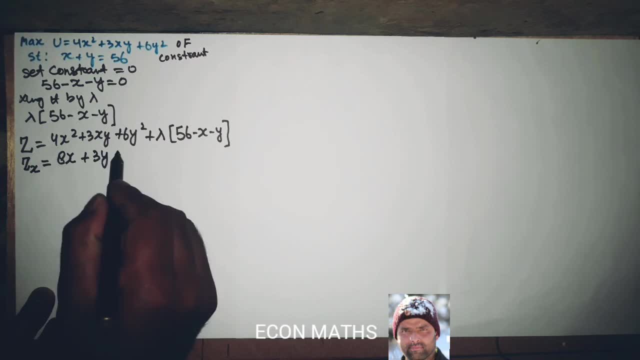 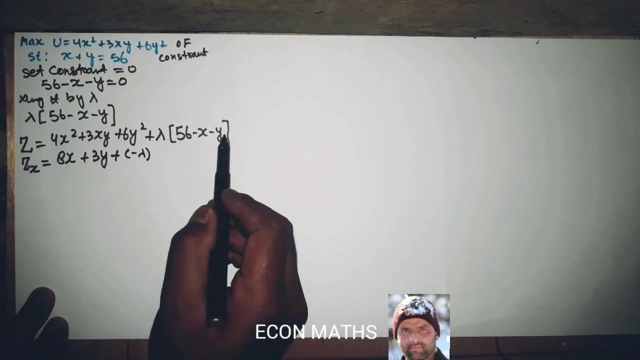 of x is 1, so this will become 3 y plus. since there is no x x involved, so it is derivative is 0. here is lambda into 56, no x involved, so it is also 0. now lambda into minus x will become the derivative of minus x is minus 1, so this will become minus lambda. now lambda into y, no x is. 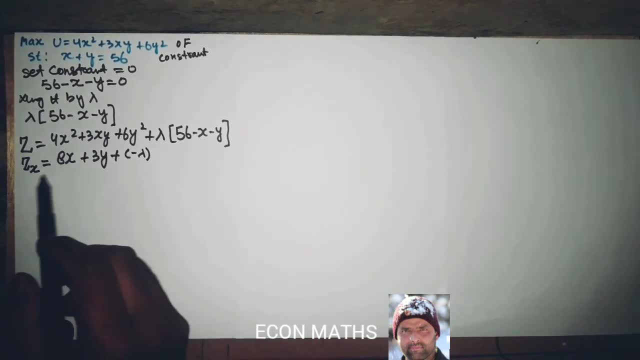 involved here, so this will also become 0. now we have differentiated this partially and we will set it equal to 0. similarly, we will differentiate with respect to y and set it equal to 0, so this is 0. that is partially differentiating with respect to y, the given Lagrange's function. so this will 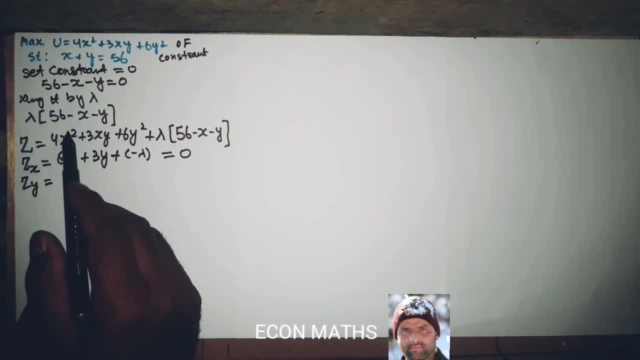 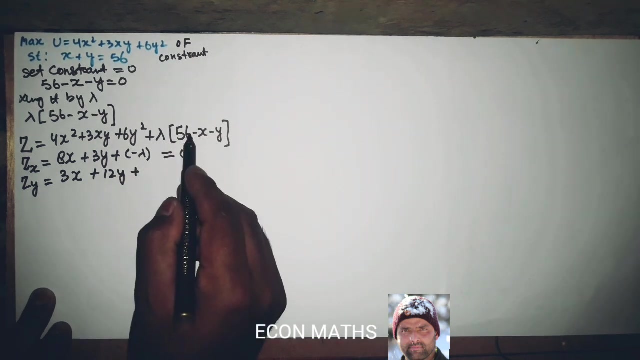 become. here no x is involved, so the derivative is 0. now here is 3 into x. into y, the derivative of y is 1, so this will become 3. x plus now 2 into 6 is equal to 12, y, similarly lambda into 56: 0. 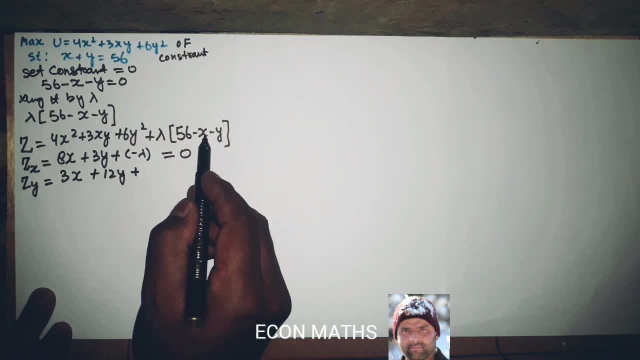 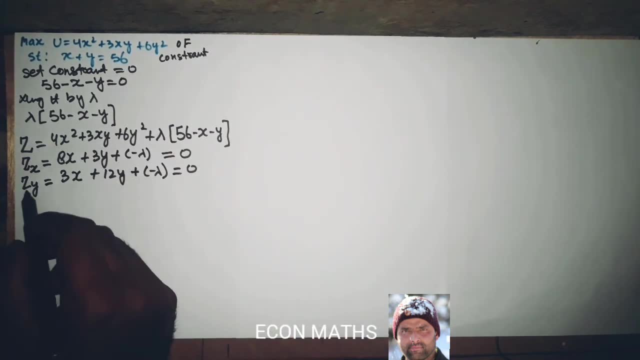 lambda into minus x, 0, because no y is involved. now lambda into minus y will become lambda. now we will equate also this to the 0, now similarly partially differentiating with respect to a lambda. so this will become: here no lambda involved, here is no, also lambda involved. and here: 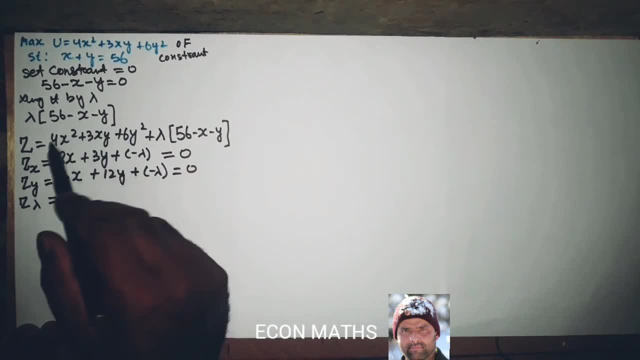 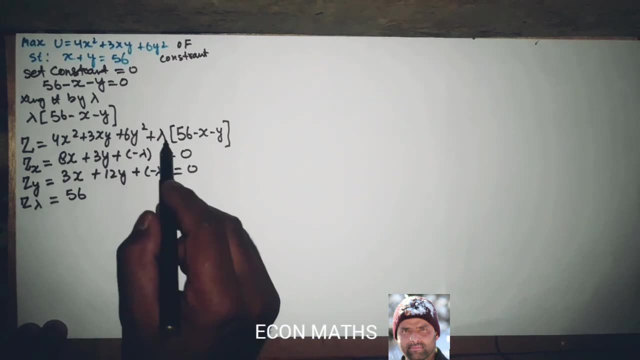 is no lambda now, so this is 0, 0 and 0. now, lambda m to 56 is 56. the coefficient, also the derivative of lambda, is 1. similarly, lambda m to minus x, the derivative of lambda is 1, so this will become minus. 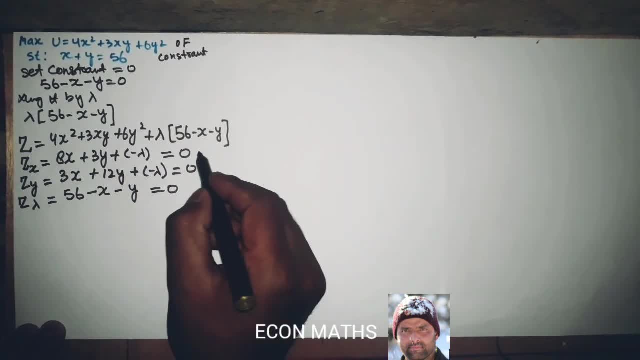 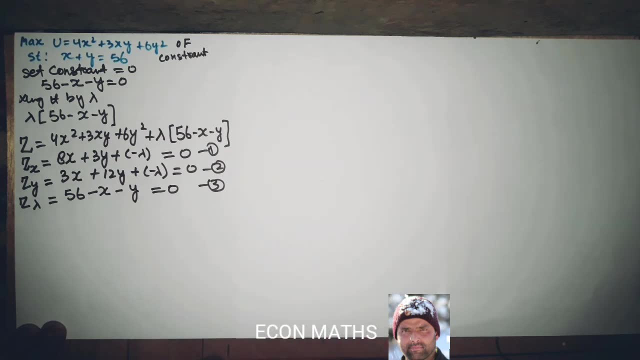 y and we will set it equal to 0. let this be equation first, second and third. we will solve these equations to get the value of x, y & lambda. now we will. we will subtract equation second from 1, so actually two equations. second from one will give us now 8 minus 3. is 4 u X per U X, now 3 minus. 12, 3 minus do, L is number two, function menosзyba, and let this be the second equation, 0 and we solve this white product. that is not true, because we do not know the sum of these equations. we can add them together. towers. 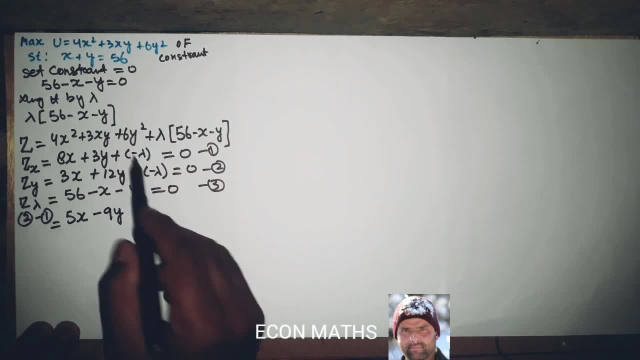 minus 9y now minus into minus, into minus into minus. so this will become plus lambda, minus lambda. minus minus plus. so minus lambda plus lambda will cancel each other, so this will: this is zero. now solving this: x is equal to x is equal to 9, y our 5.. now we will put this value. 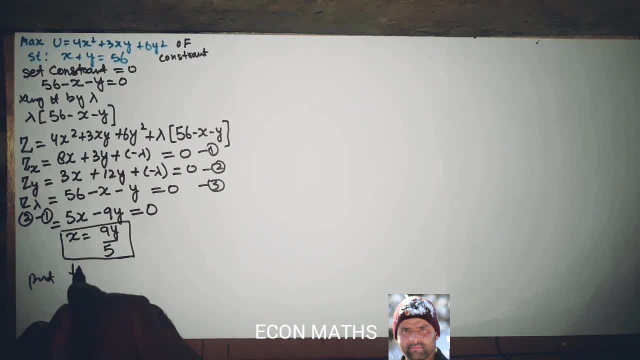 put the value of x in equation. third, we will put the value of x in this equation, so this will become 56 minus now x. we will write in x. at x, we will write 9 y. our 5 minus y is equal to 0. now solving this. solving this will give us this will become 50 seconds minus 2.8 y. 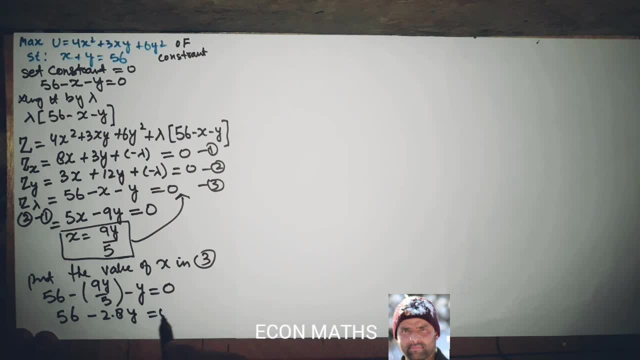 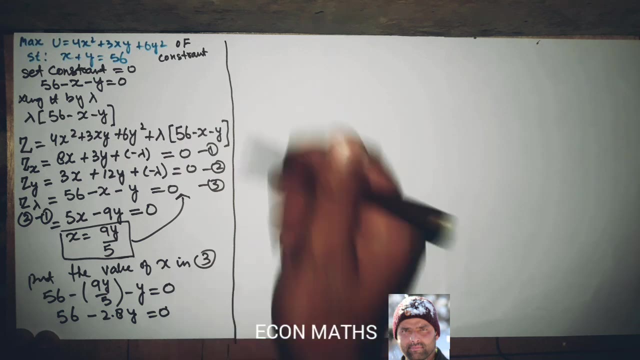 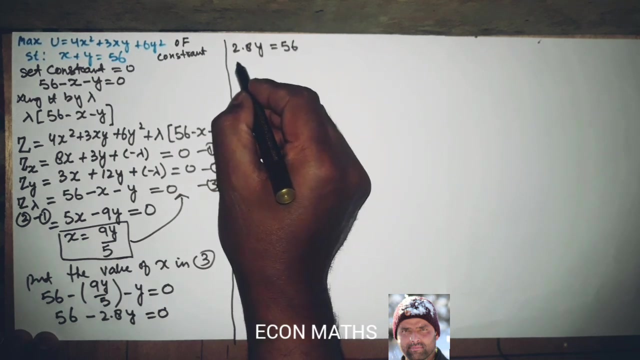 2.8 y is equal to 0. now again, solving this. i am skipping some steps because of the lake of the space, so this will get uh lengthy. if i write all the steps- i hope you are getting the steps here now- this will become 2.8. 2.8 y is equal to 50 seconds, or y is equal to 56. our 2.8, that is y is equal to. 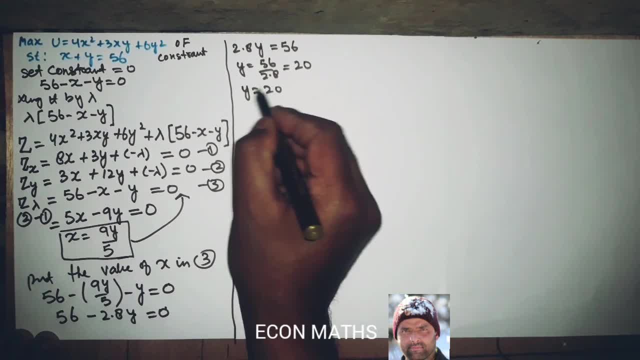 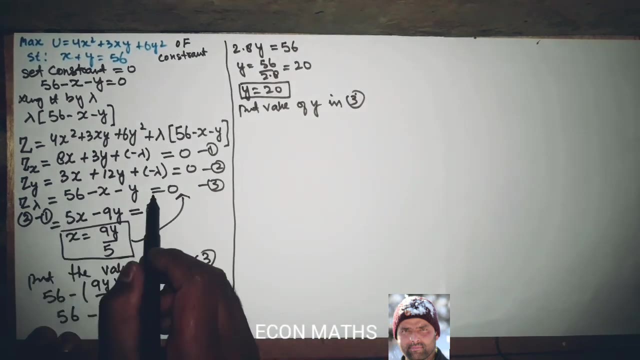 20.. so value of y is 20.. now we will put the y value of y in equation third. put value of y in the equation third. so our equation third is: this is 50 seconds minus x. minus 20 is equal to zero. now solving this and this will become: this will become minus x. now transposing: 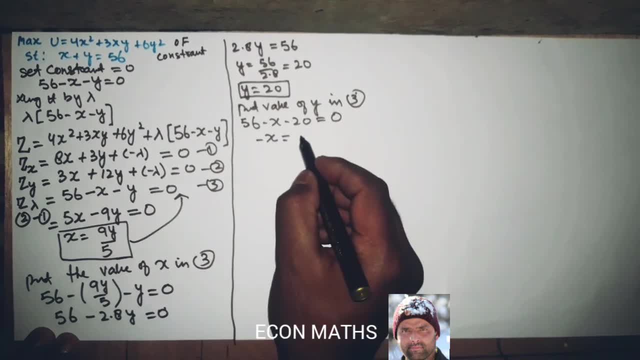 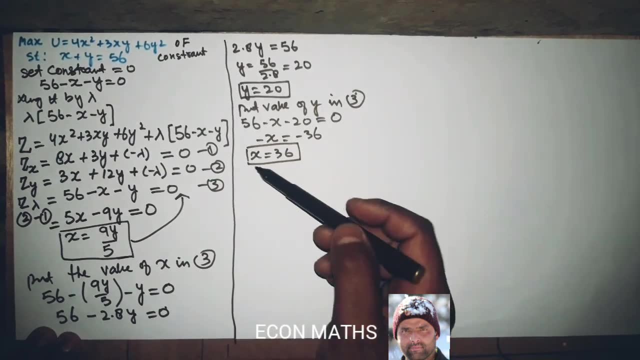 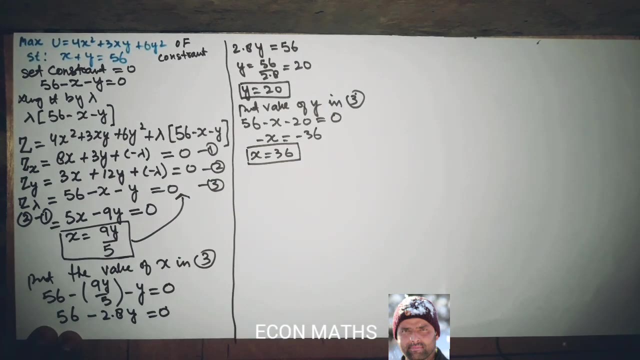 56 minus 20 is 36, and this will become minus 36, or x is equal to 30 seconds. so this, this is the value of x. now put the value of x and y in either of the two equations, because here lambda is involved. we can easily get the value of lambda now put: 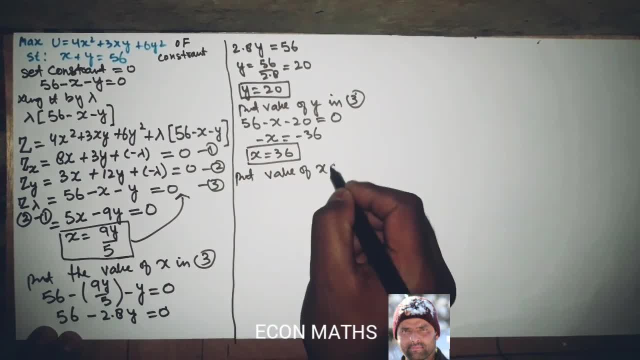 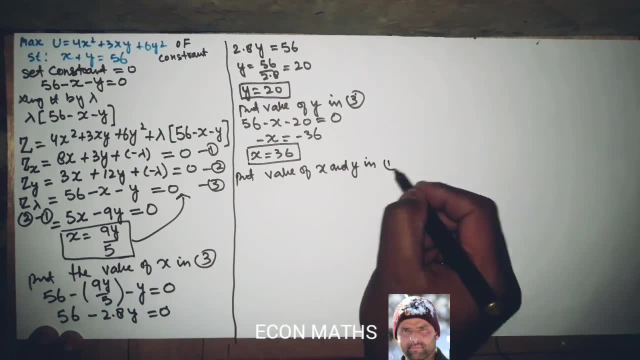 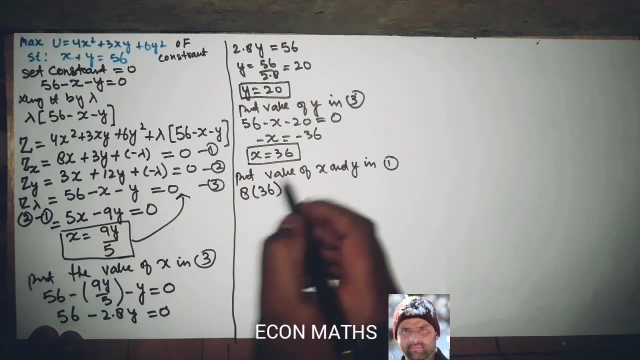 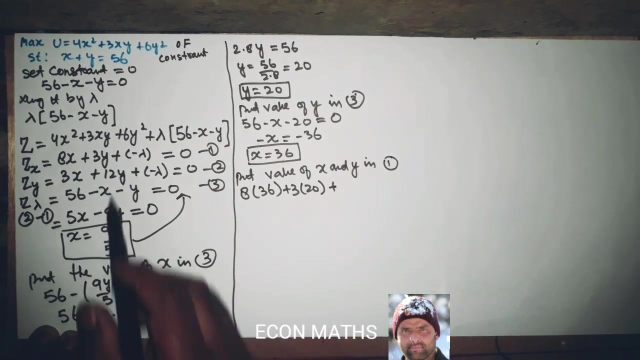 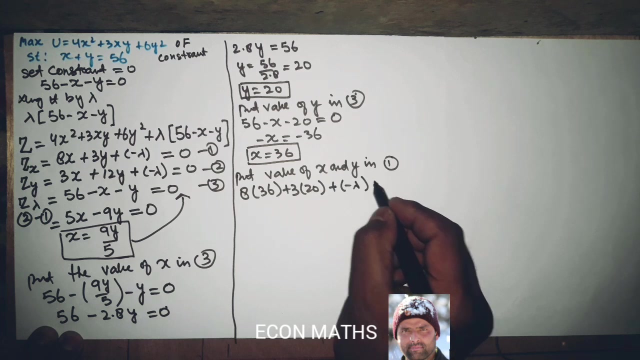 put value of X and Y in either in equation 1 or 2, so we will put it equation first. so here it is 8 into X. the value of X is 36 plus 3 by the value of Y is 20 plus. here it is minus lambda. this is equal to. this is equal to 0. now. 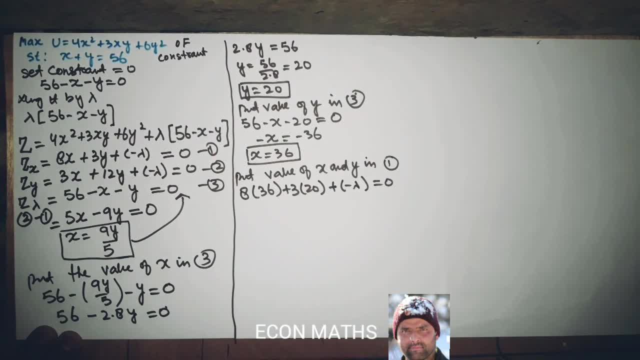 when solving this, this will become. this will become: 288 plus 60. minus lambda is equal to sorry. sorry is equal to 0. now, now again, this will become 348. assumption: minus lambda is equal to 0.. Now, minus lambda is equal to minus 348, or lambda is equal to 348.. 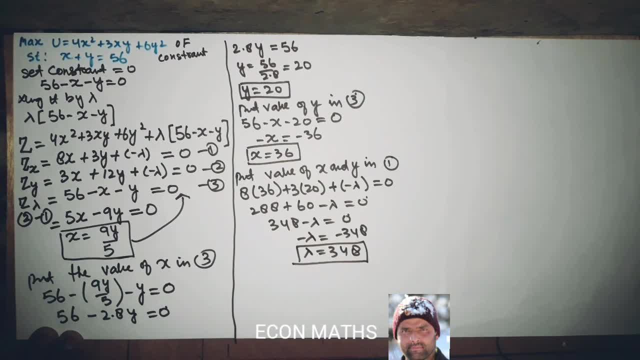 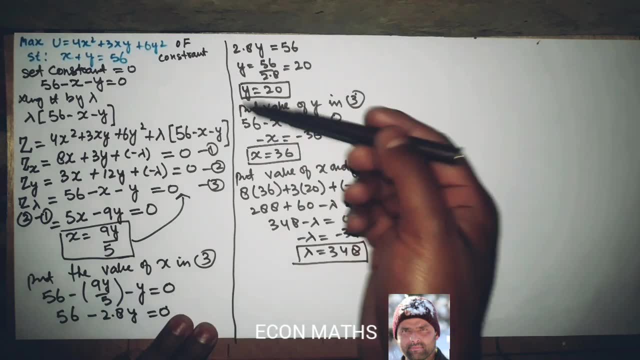 Now we got the value of lambda. Now, after that we will put the value of x, y and lambda. These are the maximum conditions, So the maximum optimal value of x and y. we got the value of x and y. 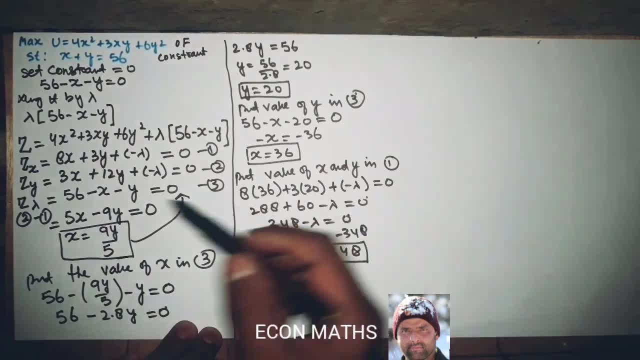 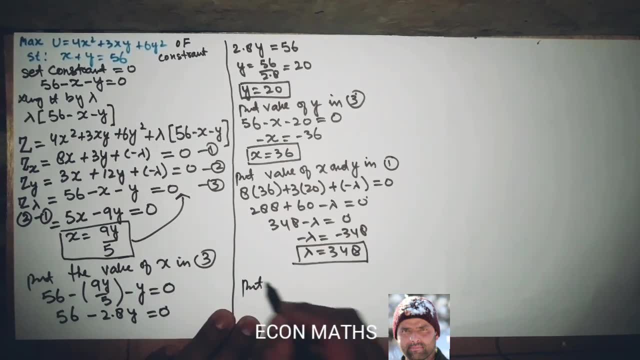 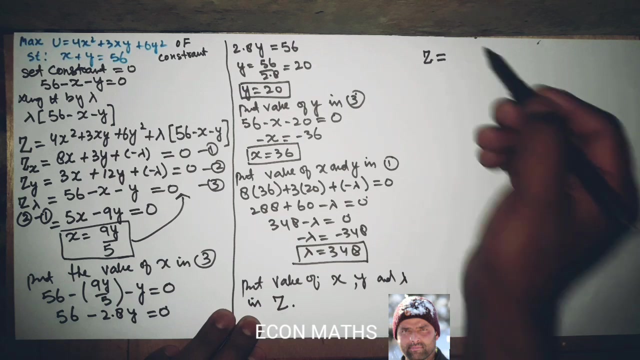 Now we will put the value of x, y and lambda in the Lagrange's function, That is, put value of x, y and lambda in z. So z is equal to z is equal to. this will become, here it is, 4,. 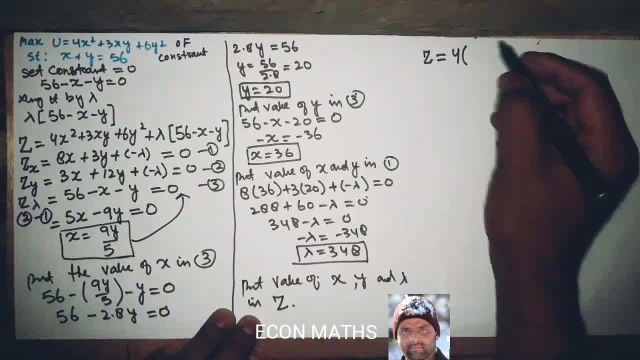 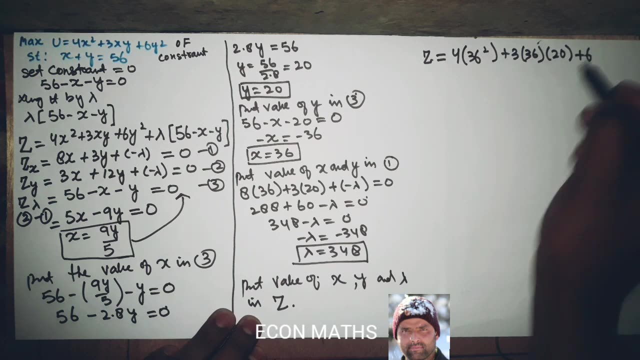 into now. value of x is 36.. Now it is squared. I will write 36 squared plus 3 into 36, and the value of y is 20.. So I will write this as 20.. Now plus 6 into 6, into y squared. So y squared. 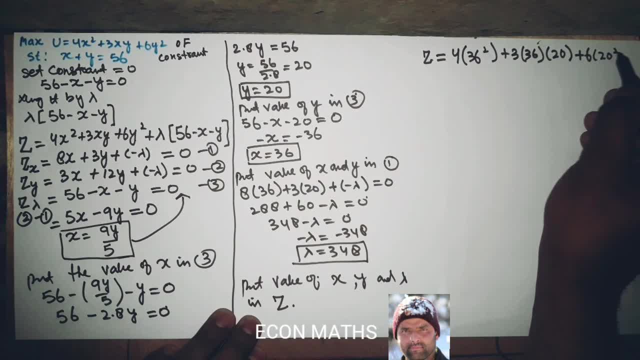 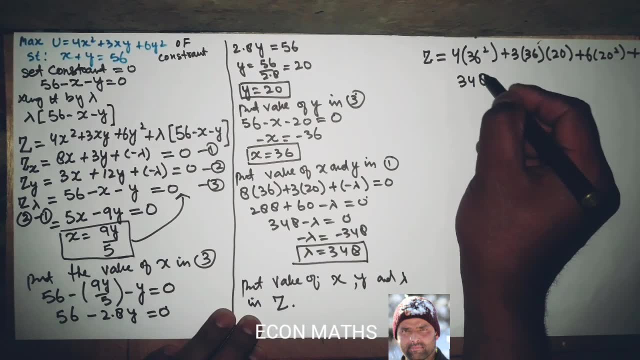 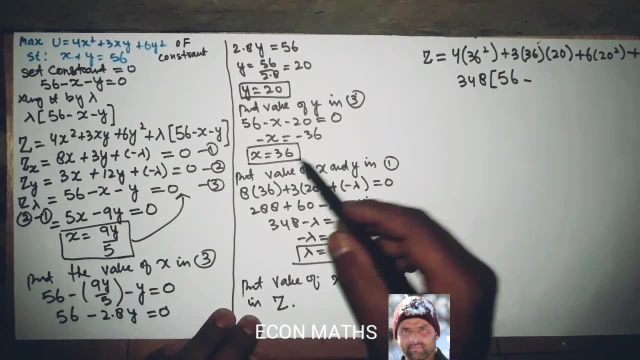 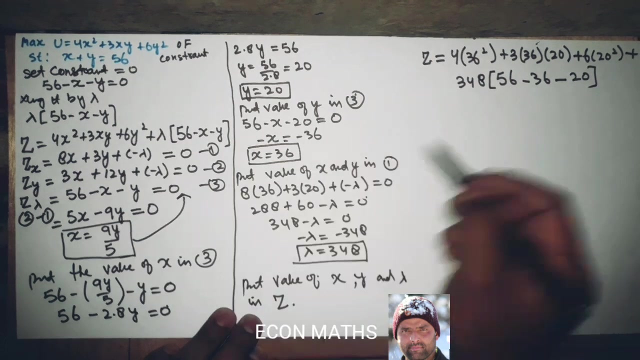 minus 20 squared. So I will write 20 squared plus lambda Lambda. we have calculated this 3, 48 into 56, minus the value of minus x. That is 36 minus 20.. That is the value of y Now. 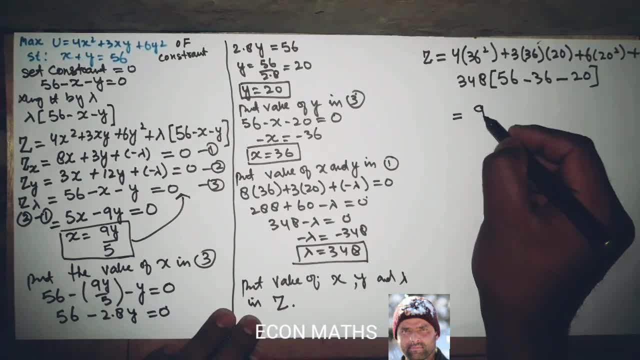 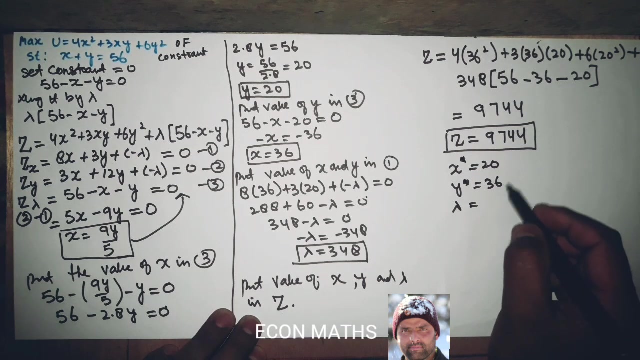 when solving this, we will come out to be 9744.. So the value of z is 9744.. And our optimal value of z is 9744.. And our optimal value of x is: value of x is 20.. y is 36. And lambda is 348.. 348.. Now